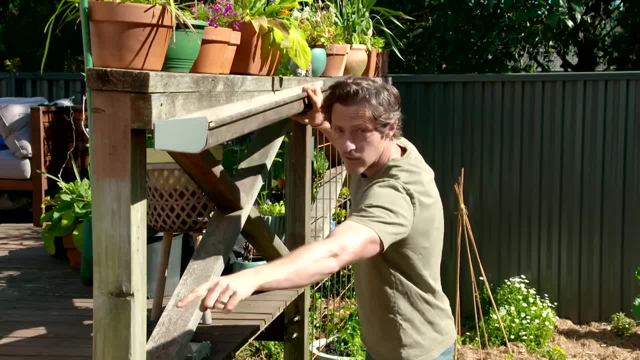 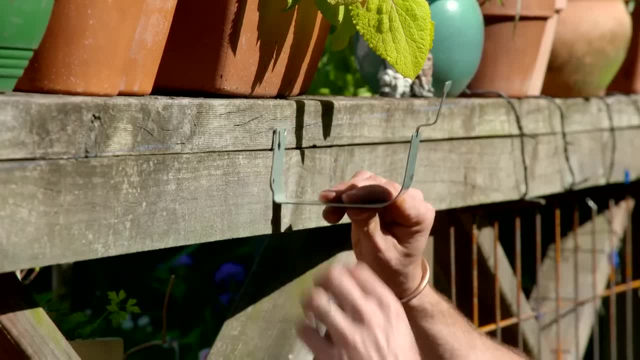 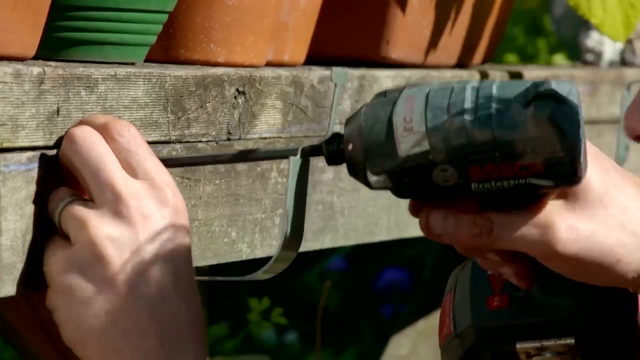 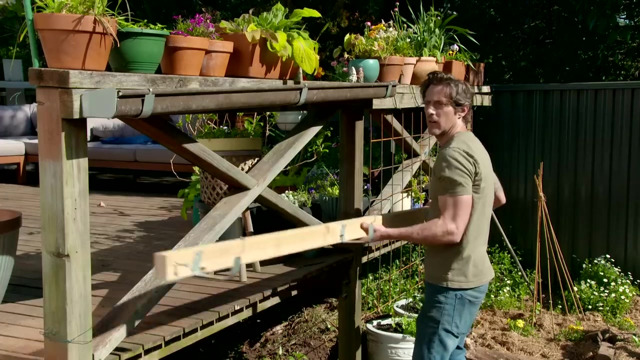 I'll have a hole in the bottom. It's going to drop into another gutter. We're going to have three gutters in total and I'm simply going to attach them to the frame using a gutter bracket like this one, Because we don't have framework across the middle of our deck. 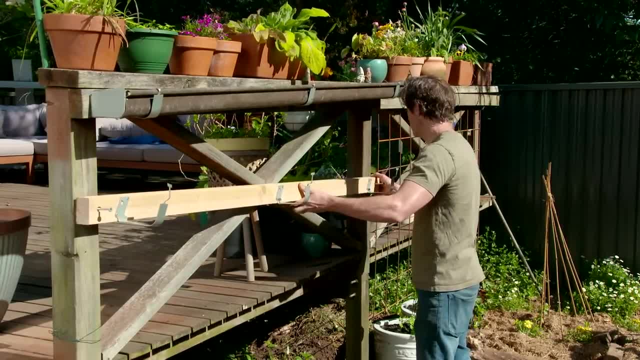 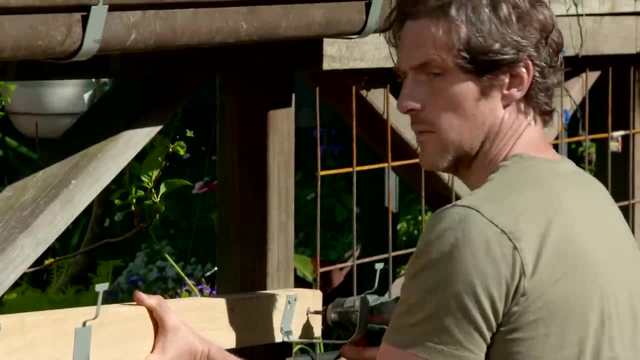 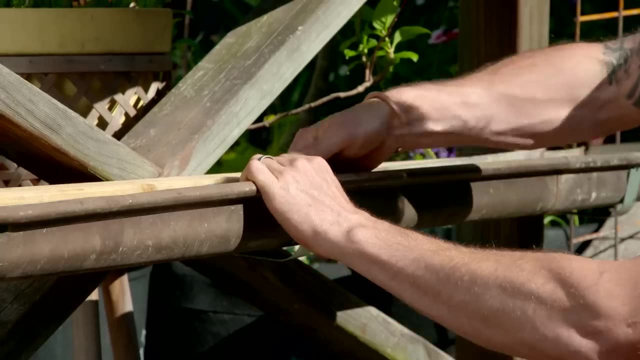 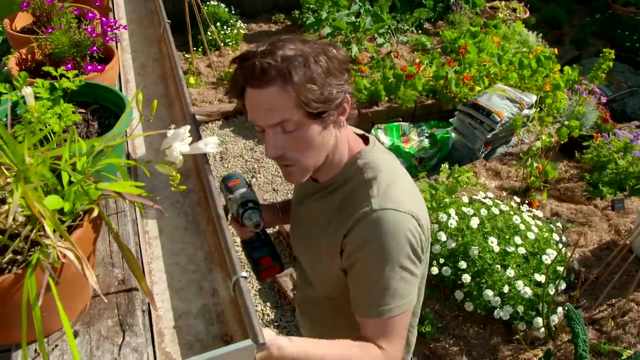 I'm just using this piece of timber that I've attached my brackets into. If you're a good hoarder, you'll have a piece of timber laying around, So I'm just going to pop some holes in the end of our gutter so the water drains through. 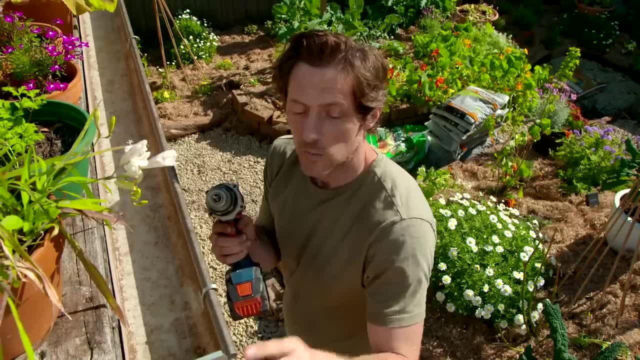 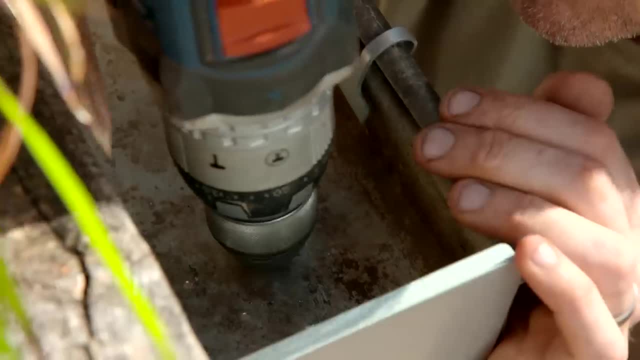 You don't want anything too big. I'm just using the same drill bit that we did the pop rivets with, but I'm going to put in three small holes. I'm just putting a bit of geotextile over the holes to stop them from clogging up, and then we can get on to the planting. 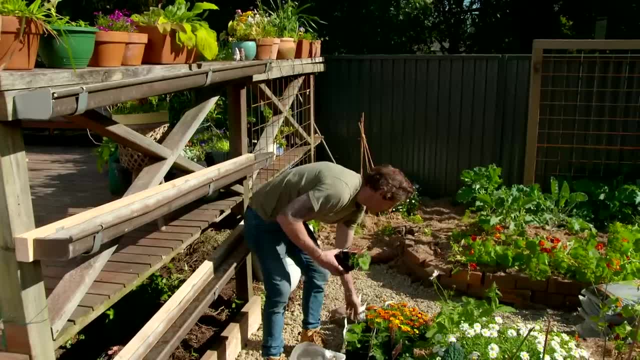 Now, I said I was going to use strawberries, but I'm also going to use some marigolds as well. When it comes to planting hydroponically, you want to try and get the soil off the ground. The best way is to shake it. 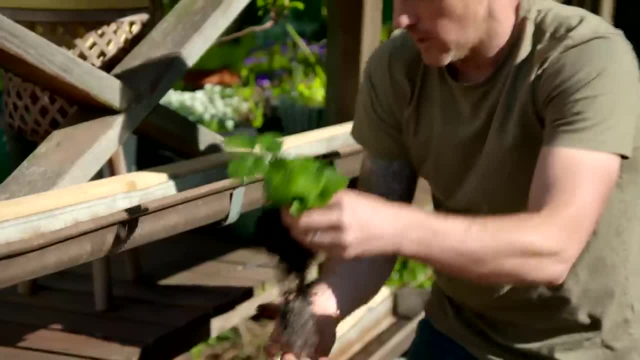 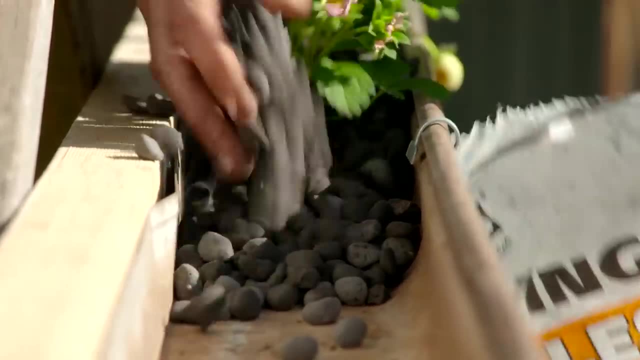 You don't want to be touching the roots too much because you can damage them. You pop it into your gutter, like so, and then backfill with some clay balls. Now, these are nice and lightweight. You use them in hydroponics because roots can get out into them. 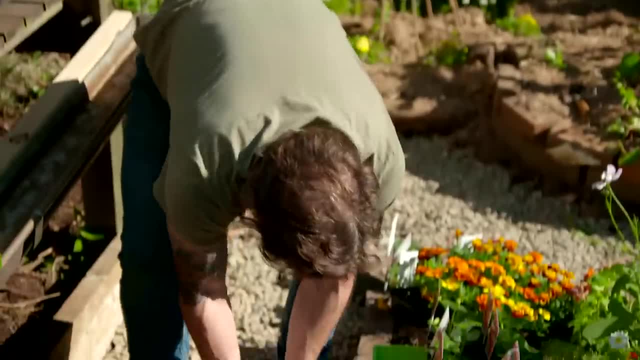 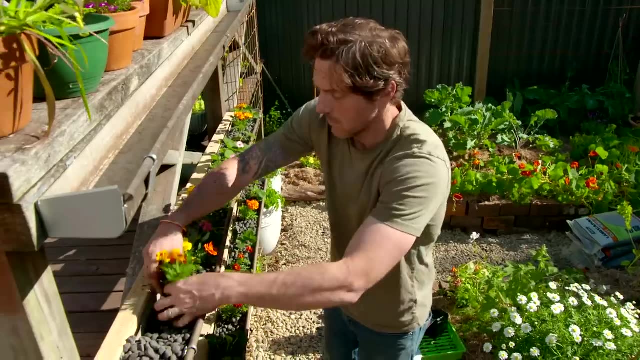 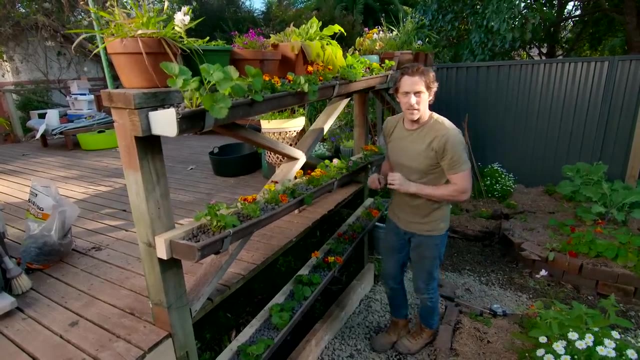 but water can flow between them as well. perfectly With the plants in, we're missing one vital ingredient to turn this into a hydroponic setup, and that is water. So I have a plastic pot here which we're using like a pond. 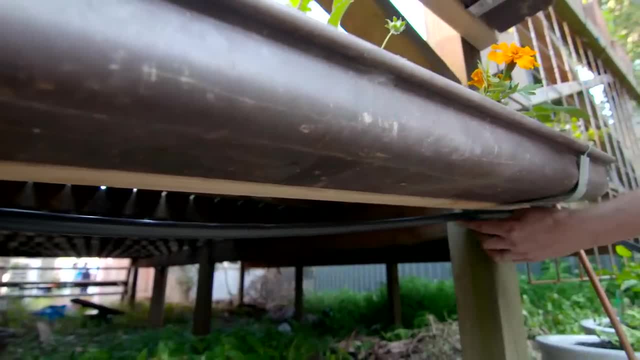 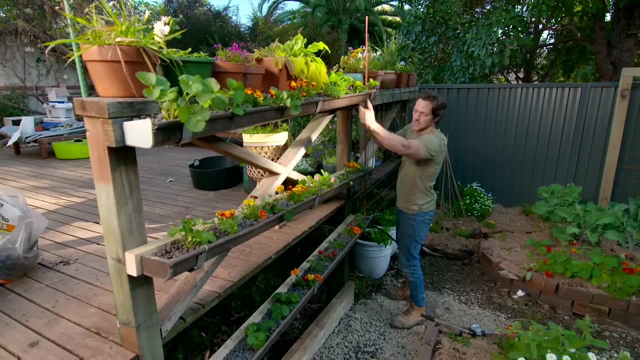 I've got a pump in it and we're just pumping water all the way up here to this copper pipe, which I will then bend over into the top, and it's going to recirculate all the way through and give the plants exactly what they need.